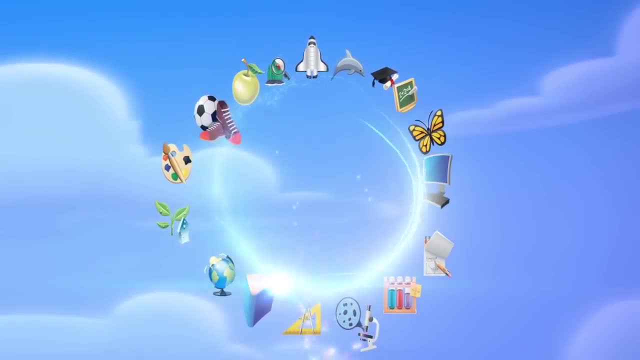 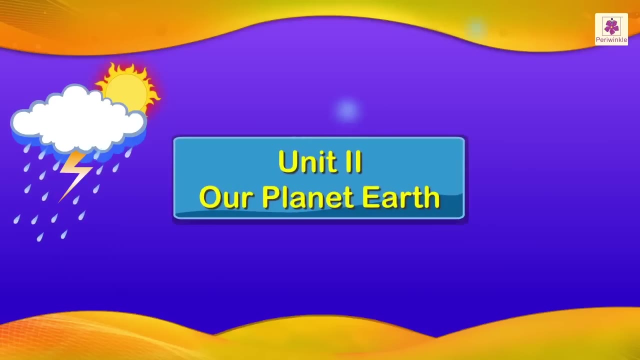 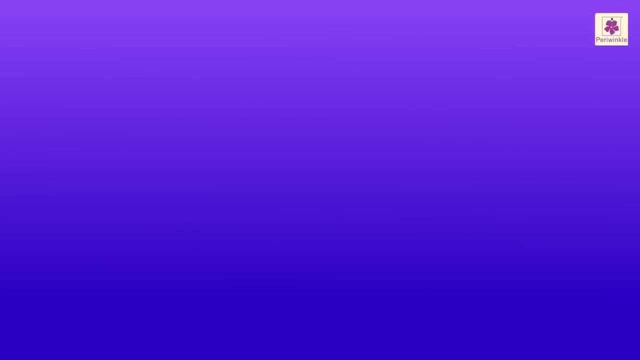 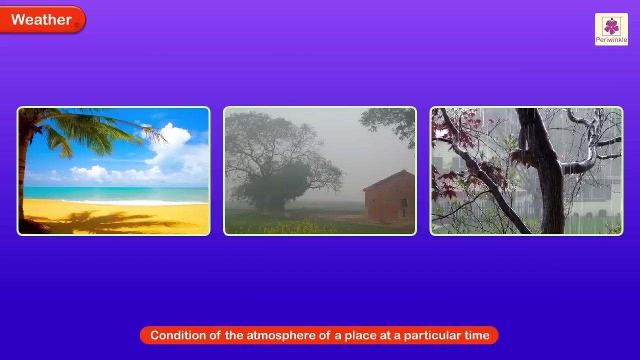 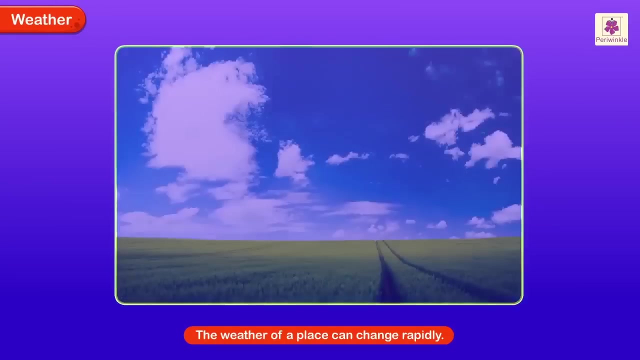 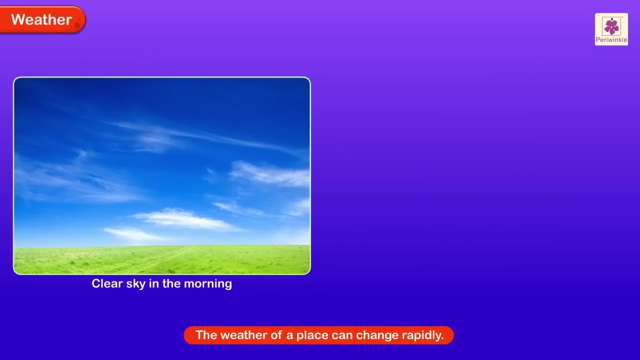 Unit 2: Our Planet Earth Weather and Climate Weather. Weather is the condition of the atmosphere of a place at a particular time. The weather of a place can change rapidly. It may be bright and sunny, with a clear sky in the morning, while in the evening the sky may be covered with dark clouds. 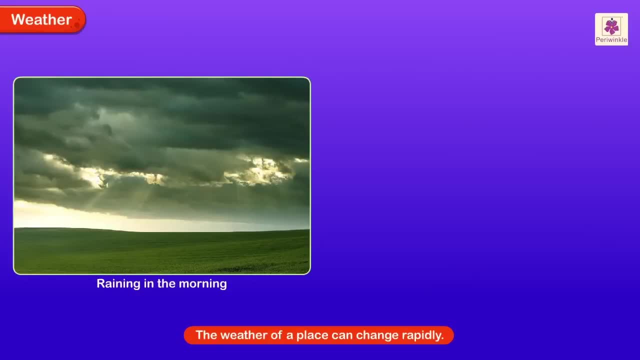 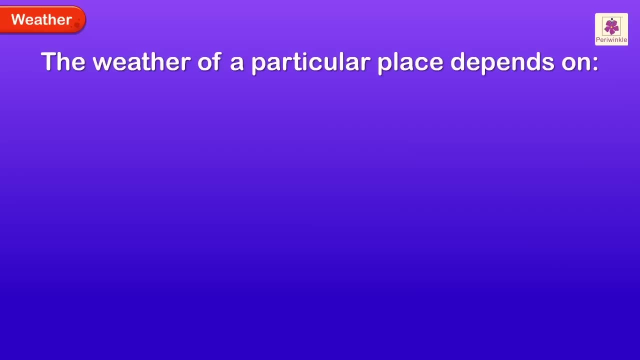 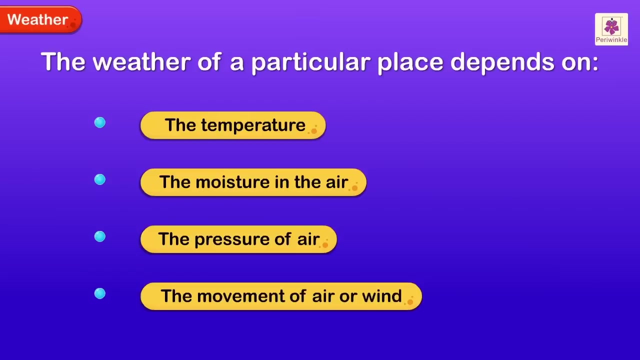 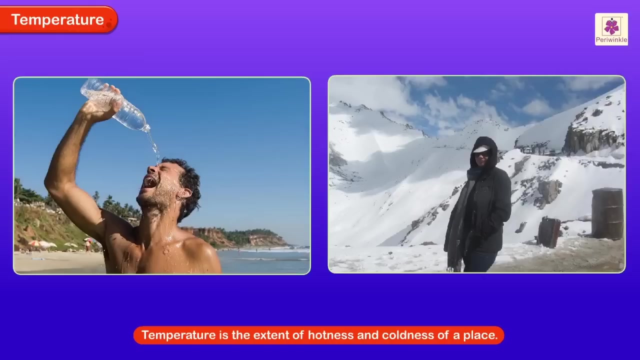 It may start raining in the morning, but the afternoon may be bright and sunny. The weather of a place can change rapidly: The temperature, the moisture in the air, the pressure of air, the movement of air or wind. Temperature Temperature is the extent of hotness and coldness of a place. 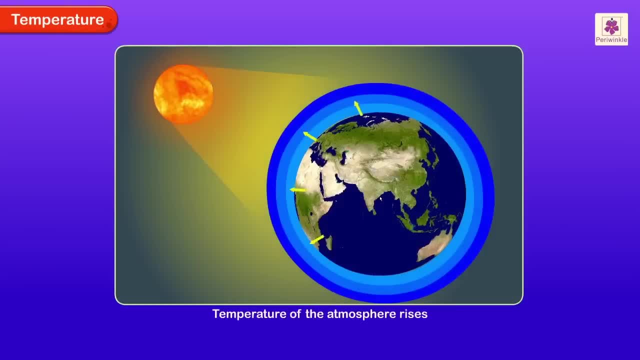 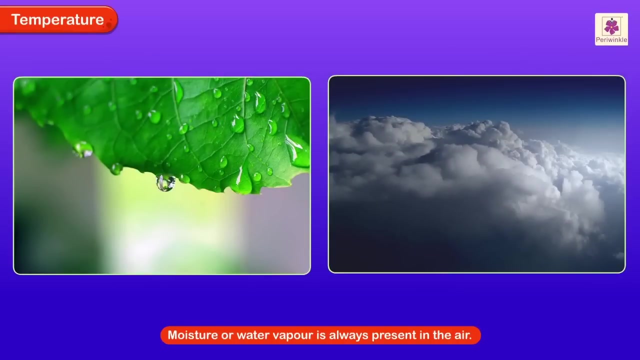 The earth gets heated by the sun. As the sunlight reaches the earth, the temperature of the air and the temperature of the air changes. The earth gets heated by the sun, The earth and the earth. liquid fuckingнев t present in the air. the amount of moisture in the air rises when the sun's 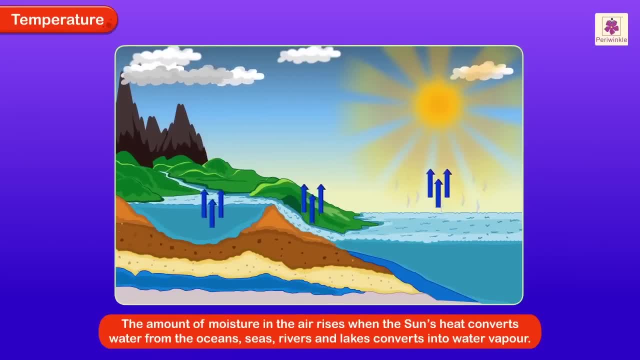 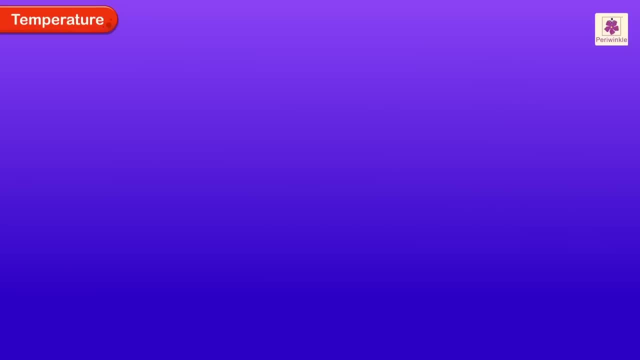 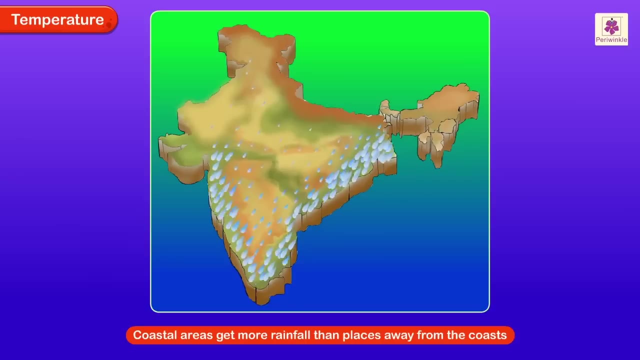 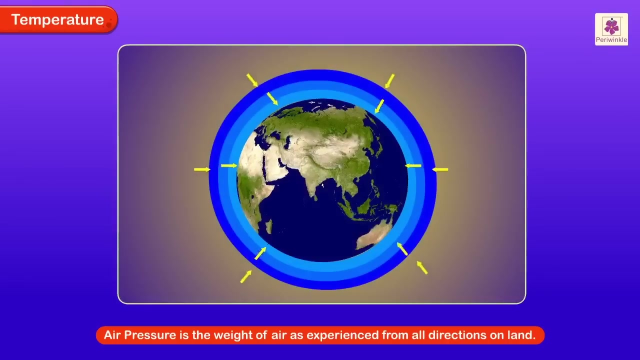 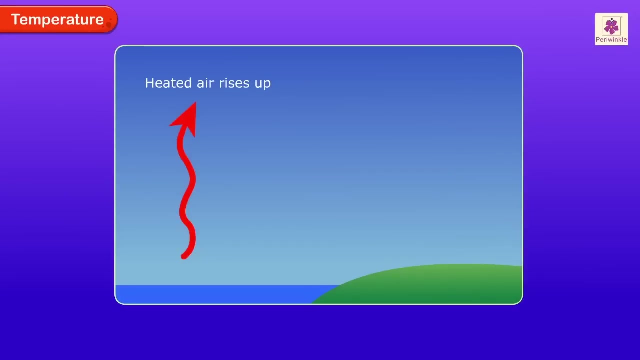 heat converts water from the oceans, seas, rivers and lakes into water vapor. this is the reason why coastal areas get more rainfall than places away from the coast. air pressure is the weight of air as experienced from all directions on land. when air heats up, it rises and creates an area of low pressure on the earth's. 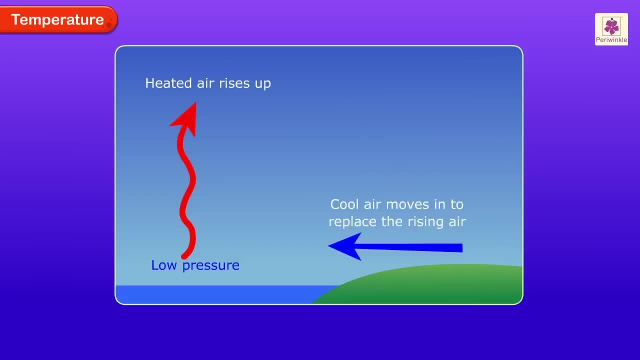 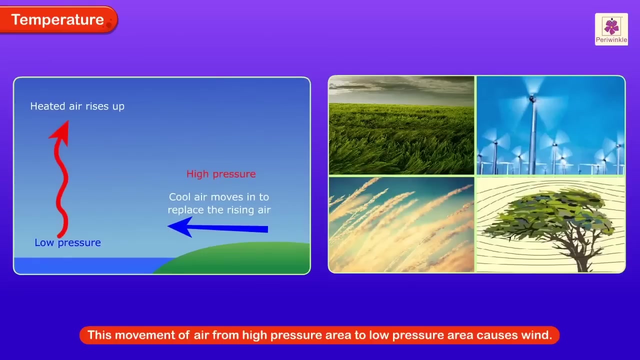 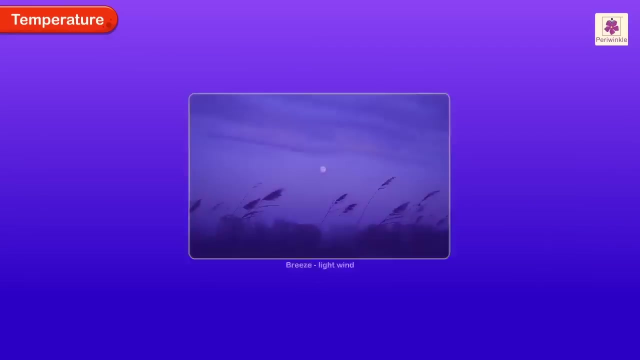 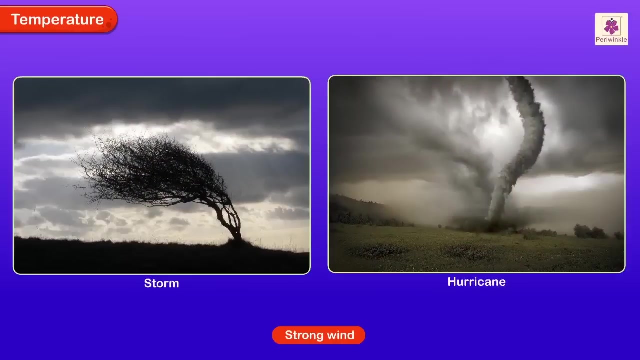 surface. the surrounding cool air moves in to replace this rising air. this air comes from areas where the pressure is high you this movement of air from high-pressure area to low-pressure area causes wind. the wind is sometimes a light, pleasant breeze. at other times it can be very. 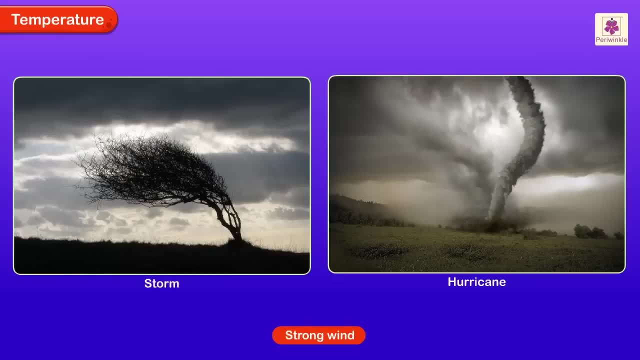 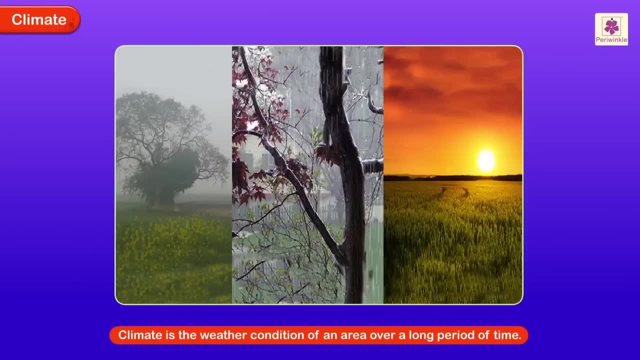 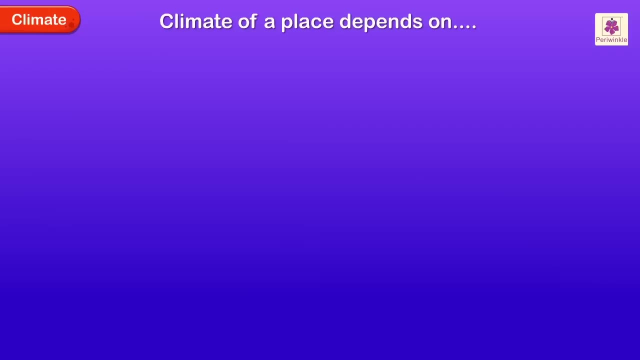 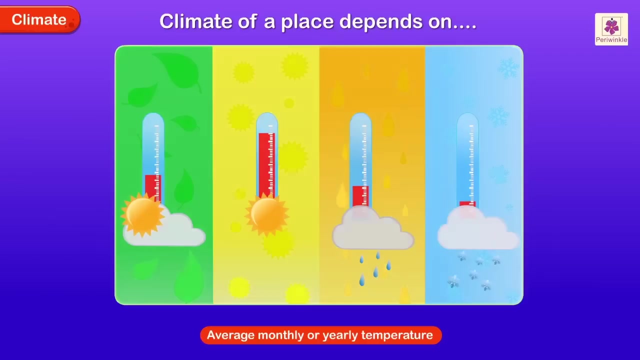 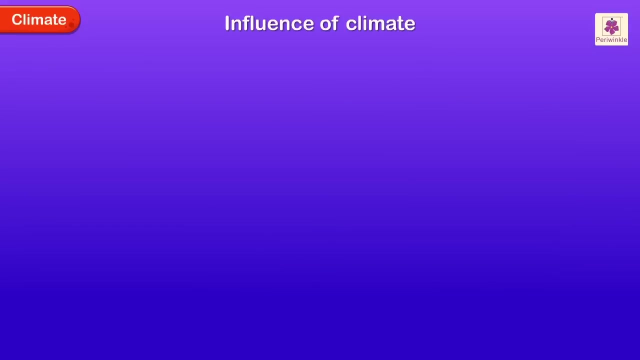 strong and can cause a storm or a hurricane. climate climate is the weather condition that causes the air to move from high pressure area to low pressure area. climate of a place depends on its average monthly or yearly temperature. average amount of rainfall or snow. climate influences the type of food. 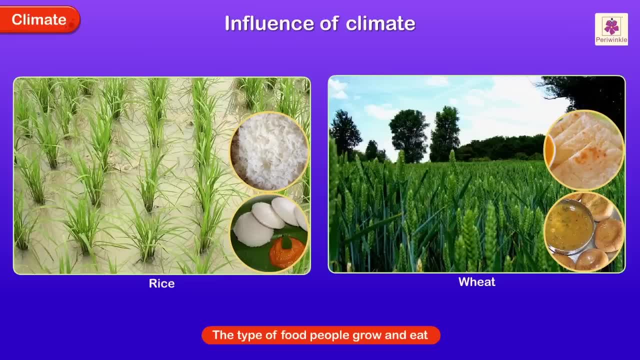 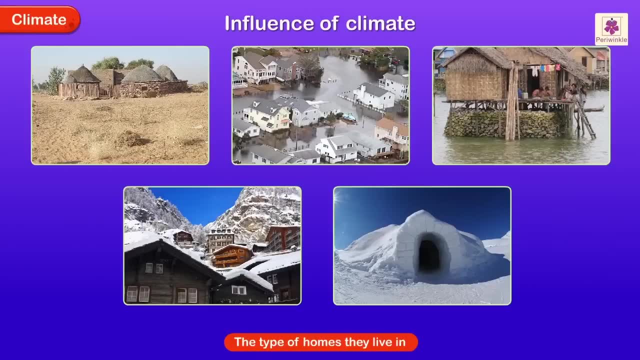 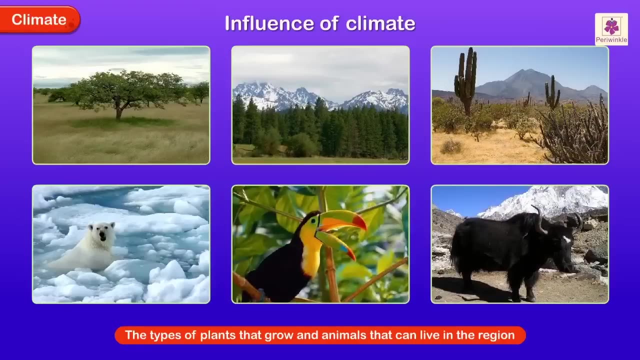 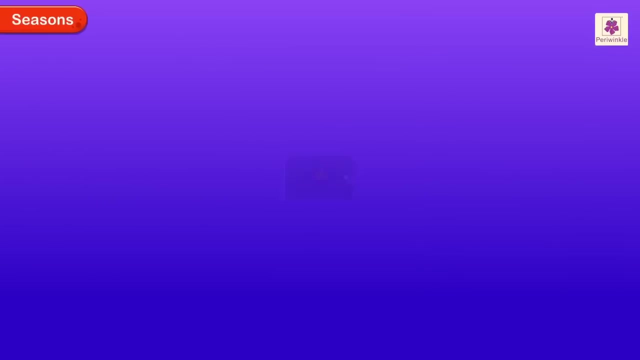 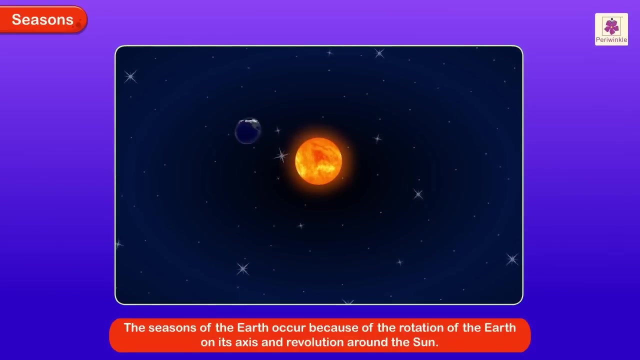 people grow and eat. climate influences the type of food people grow and eat, the type of clothes they wear, the type of homes they live in, the types of plants that grow and animals that can live in the region. seasons: the seasons of the earth occur because of the rotation of the earth on its axis and revolution. 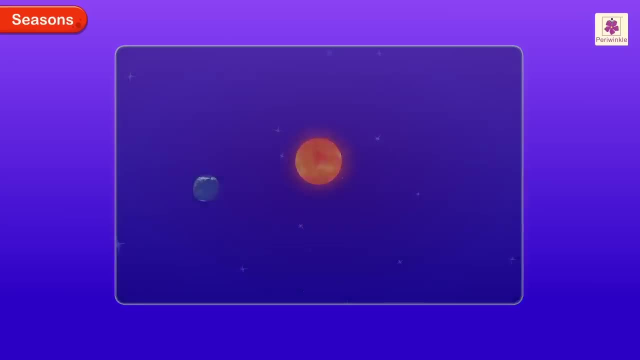 around the Sun. the seasons of the earth occur because of the rotation of the earth on its axis and revolution around the sun. the seasons of the earth occur because of the rotation of the earth on its axis and revolution around the sun. around the sun, there are mainly three seasons in India. 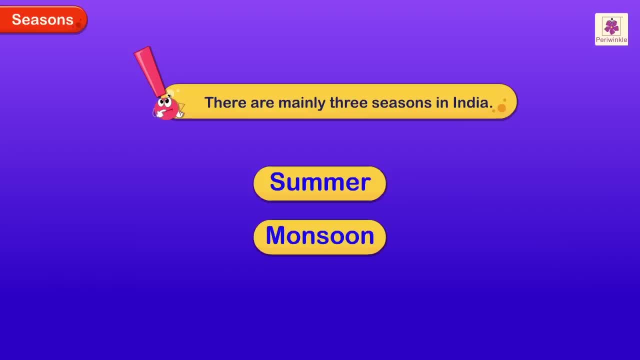 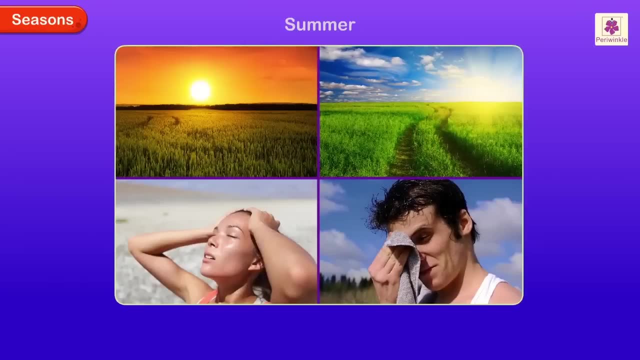 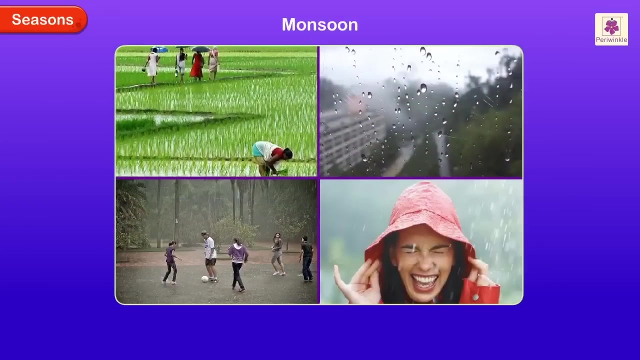 summer, monsoon and winter summer. from March onwards it grows hot. from March onwards it grows hot. March, April and me are the summer months. monsoon, month of June, March Twitter. this is a June. Rain clouds gather in the sky, bringing rain to most parts of India.